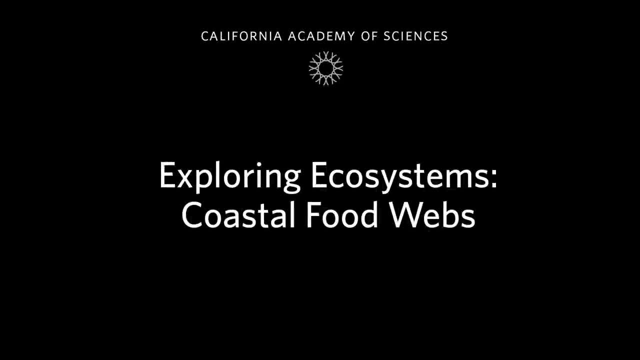 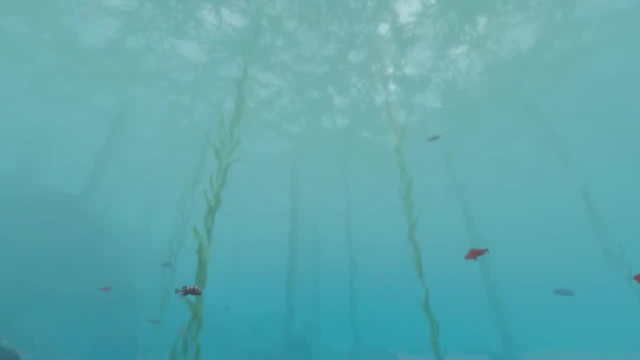 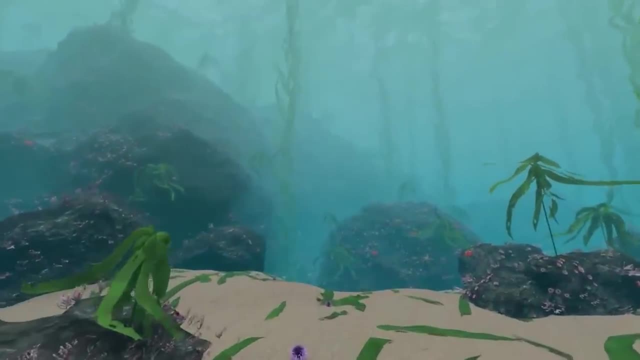 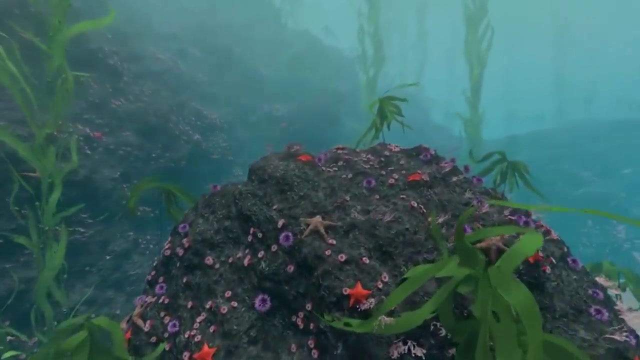 Let's visit an underwater forest near Monterey, California, where kelp grows over 100 feet tall, reaching towards the sunlight above Its. fallen blades litter the seafloor below, providing nutrients for a host of creatures, including these spiny purple sea urchins. 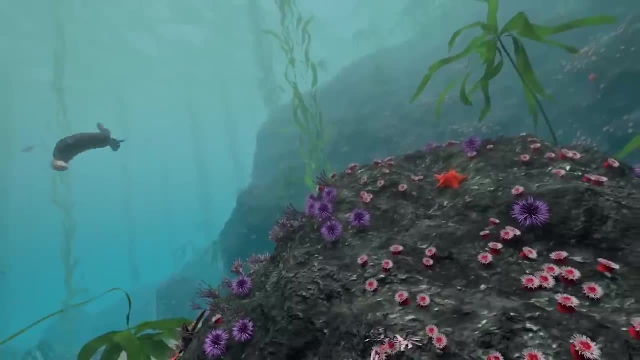 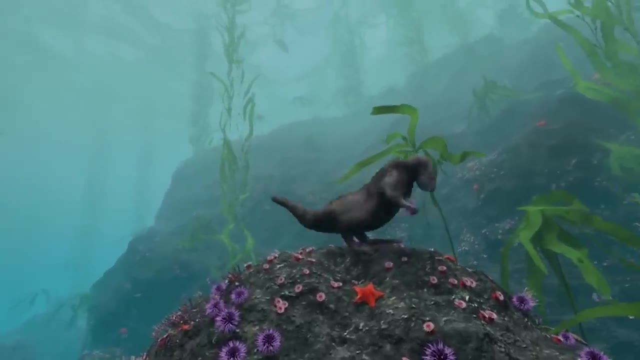 which move slowly in search of food. Sea urchins make a tasty meal for this marine mammal. Sea otters help keep the sea urchin population in check. Too many sea urchins will devour living kelp, destroying the forest. 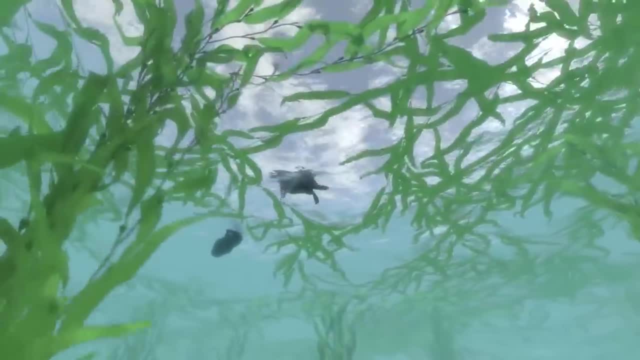 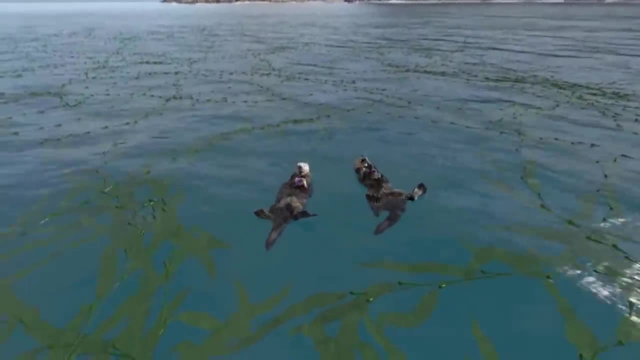 We consider otters a keystone species. As active predators, they protect kelp from hungry herbivores like sea urchins and help maintain diversity and balance in this ecosystem. But we're seeing just one of the most interesting things about kelp. It's one small part of an intricate network. Sunflower stars also prey on sea urchins and may become dinner for a hungry sea otter, But otters prefer abalone and crabs. From the smallest microbes to the largest animals, these species take part in a diverse 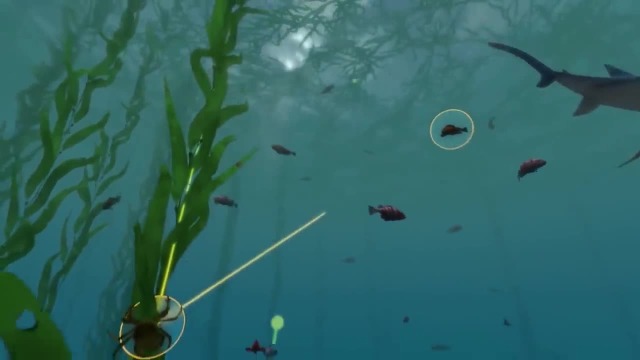 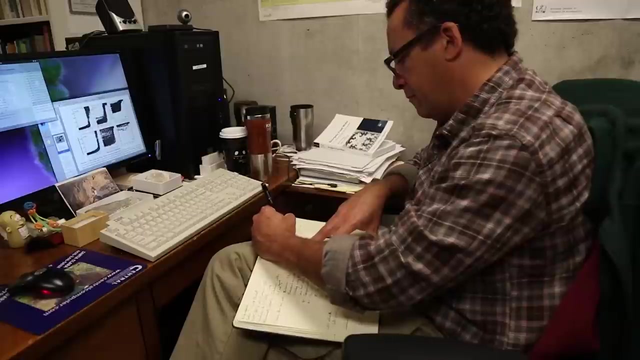 food web that links more than a thousand species. The connections in the web represent the transfer of energy with every meal. At the California Academy of Sciences, paleontologist Peter Rupnerine studies both modern-day food webs like this one and those. 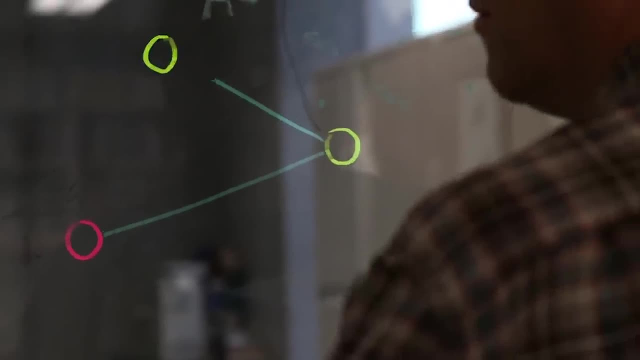 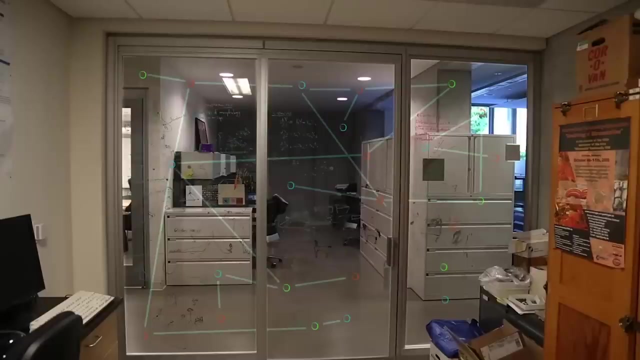 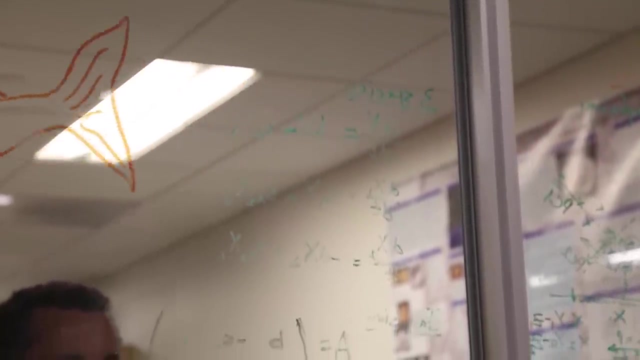 from the past. Basically, a food web is a map of all of the interactions- what we call the trophic interactions- in an ecosystem or community, And those are predator-prey interactions: Who eats whom, who eats you, what do you eat, and so on. The food web is one of, if not the most important. 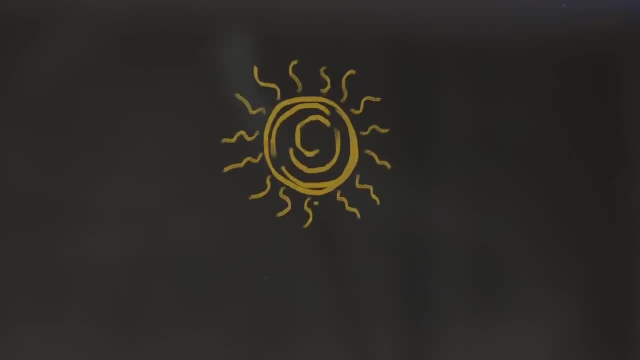 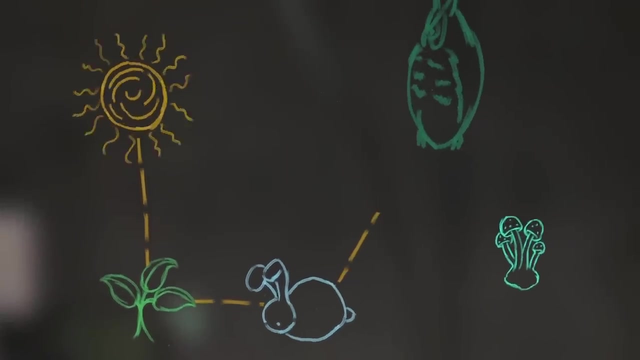 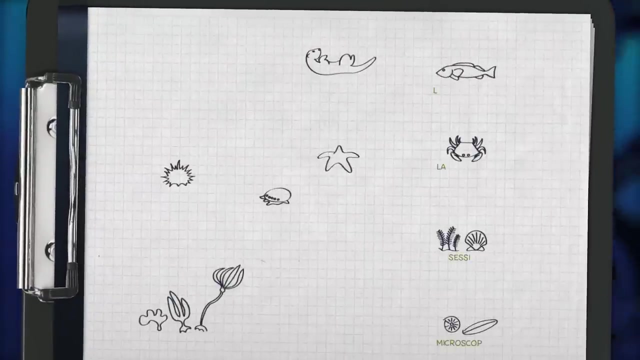 representation of interactions. It's a map of all the interactions that we have in an ecosystem, because it's a main passage of energy through that system. Energy is produced, it's consumed and everything else runs on that. Let's take a closer look at our marine ecosystem off the coast of California. What? 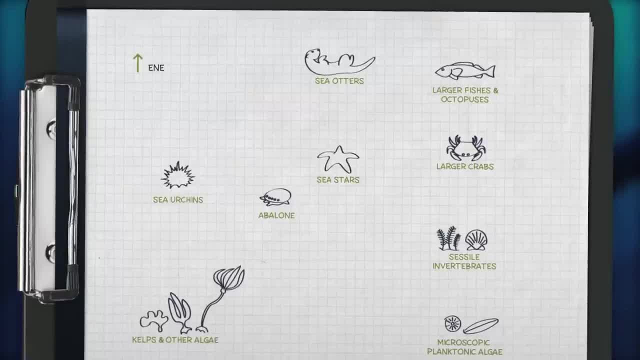 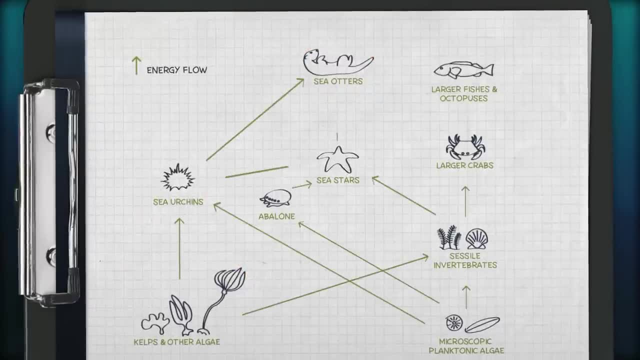 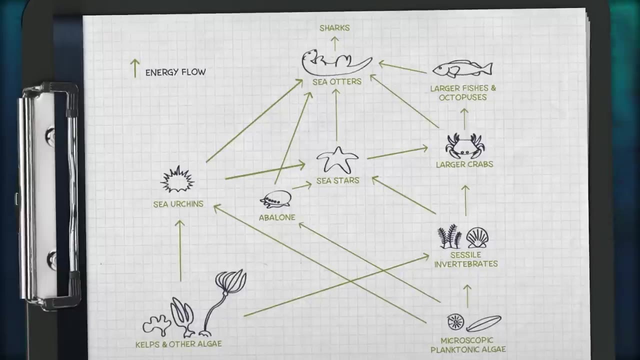 connections do you see in this food web? Can you predict the flow of energy between otters, urchins and kelp From primary producers to top predators? this dynamic ecosystem supports a diverse set of species. Small changes, however, can have big impacts across the entire community. 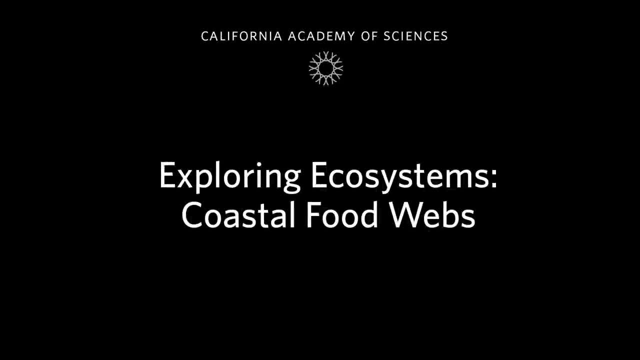 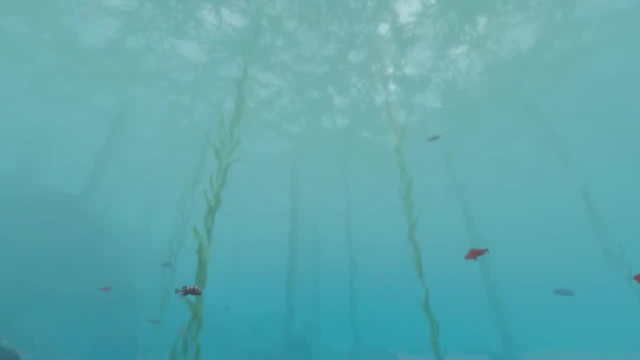 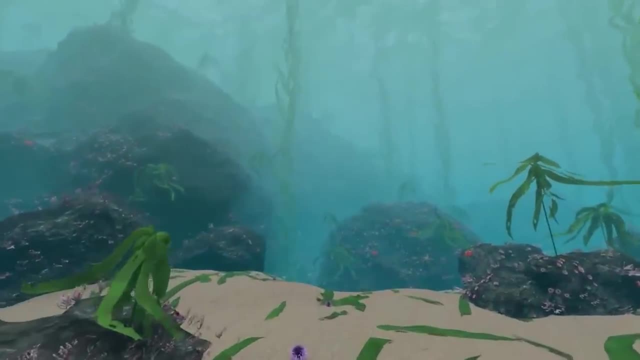 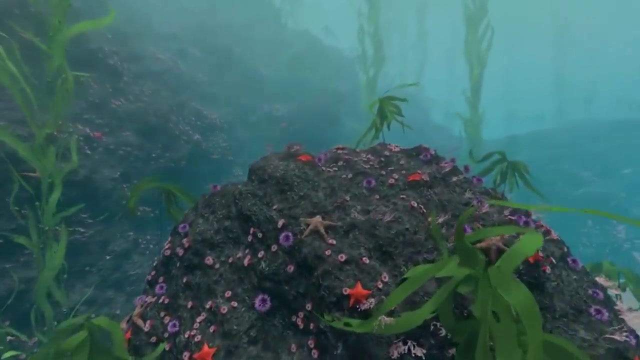 Let's visit an underwater forest near Monterey, California, where kelp grows over 100 feet tall, reaching towards the sunlight above Its. fallen blades litter the seafloor below, providing nutrients for a host of creatures, including these spiny purple sea urchins. 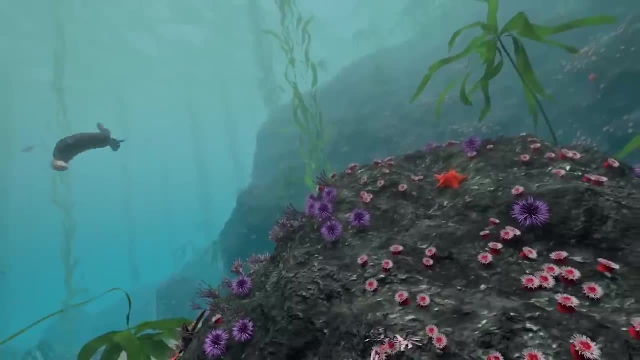 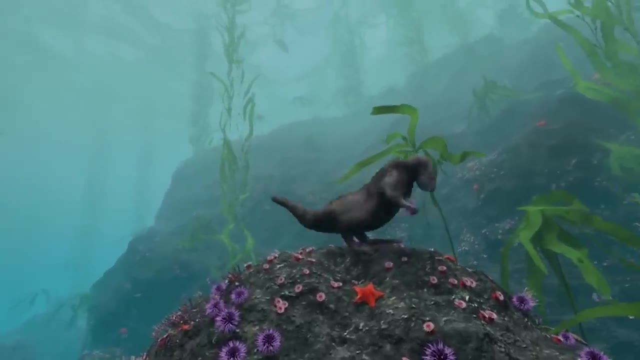 which move slowly in search of food. Sea urchins make a tasty meal for this marine mammal. Sea otters help keep the sea urchin population in check. Too many sea urchins will devour living kelp, destroying the forest. 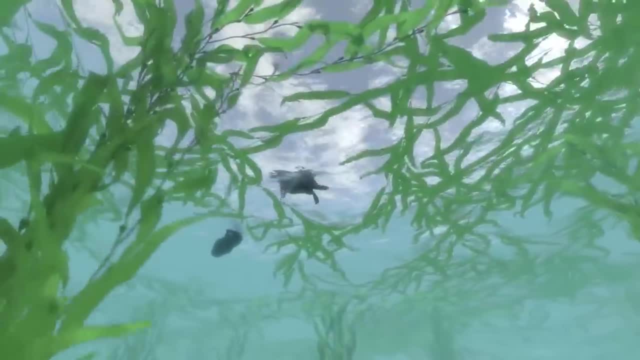 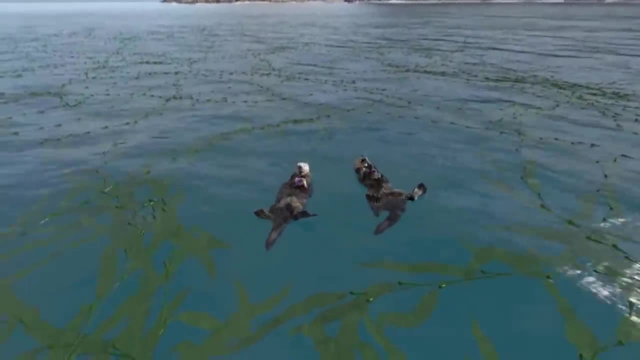 We consider otters a keystone species. As active predators, they protect kelp from hungry herbivores like sea urchins and help maintain diversity and balance in this ecosystem. But we're seeing just one of the most interesting things about kelp. It's one small part of an intricate network. Sunflower stars also prey on sea urchins and may become dinner for a hungry sea otter, But otters prefer abalone and crabs. From the smallest microbes to the largest animals, these species take part in a diverse 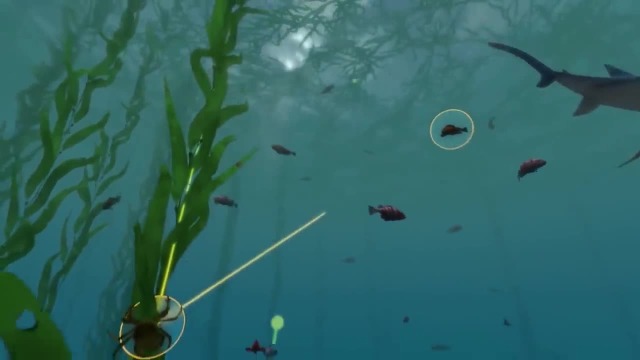 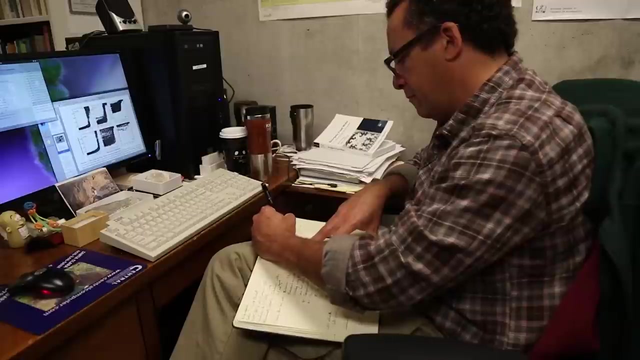 food web that links more than a thousand species. The connections in the web represent the transfer of energy with every meal. At the California Academy of Sciences, paleontologist Peter Rupnerine studies both modern-day food webs like this one and those. 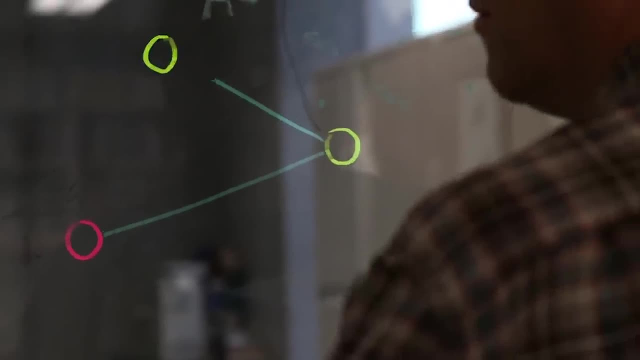 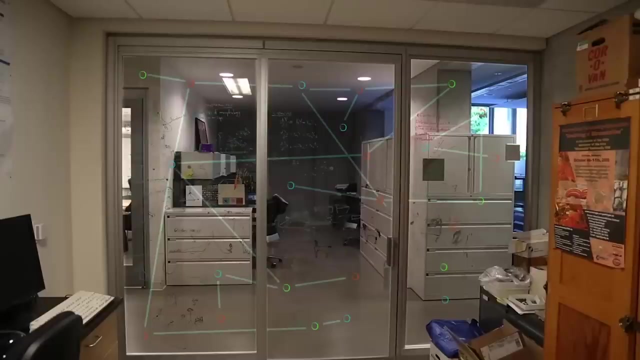 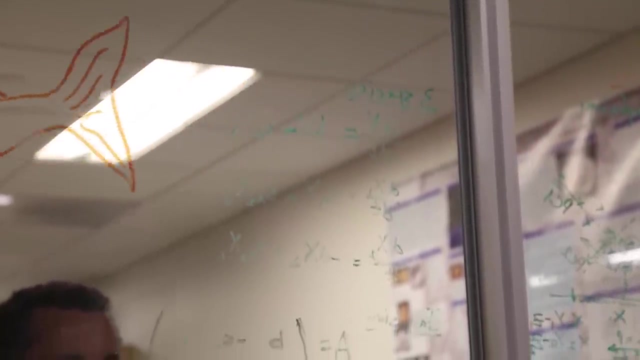 from the past. Basically, a food web is a map of all of the interactions- what we call the trophic interactions- in an ecosystem or community, And those are predator-prey interactions: Who eats whom, who eats you, what do you eat, and so on. The food web is one of, if not the most important. 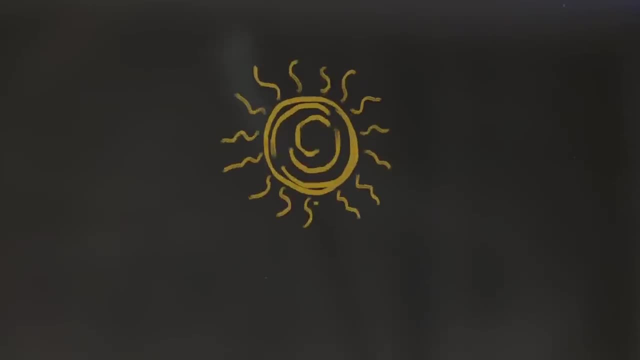 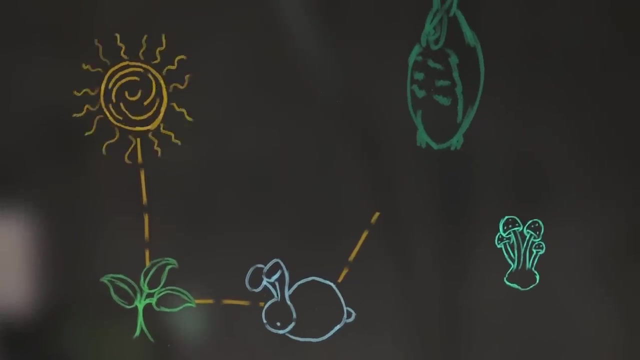 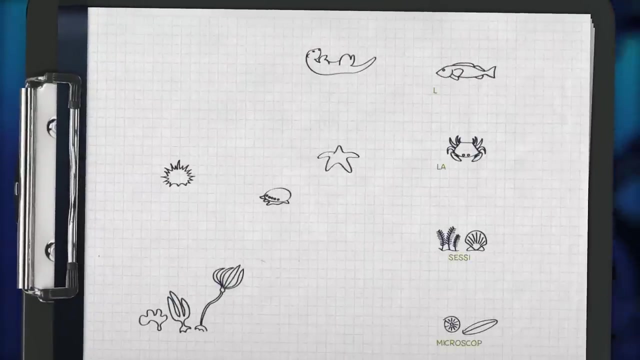 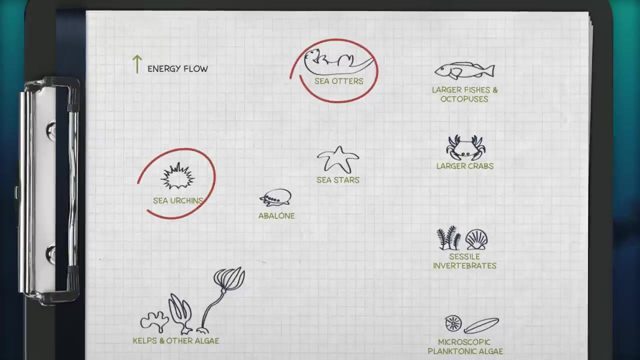 representation of interactions, Because it's a main passage of energy. through that system. energy is produced, it's consumed and everything else runs on that. Let's take a closer look at our marine ecosystem off the coast of California. What connections do you see in this food web? Can you predict the flow of energy between otters, urchins?